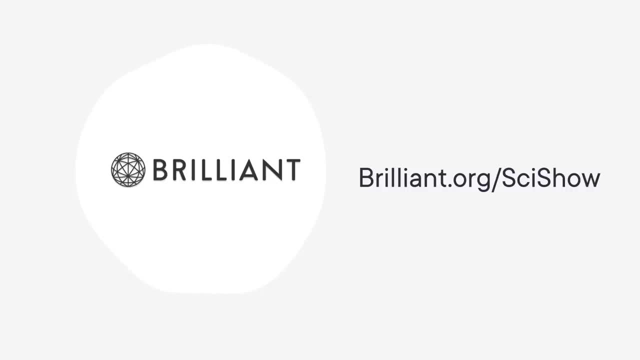 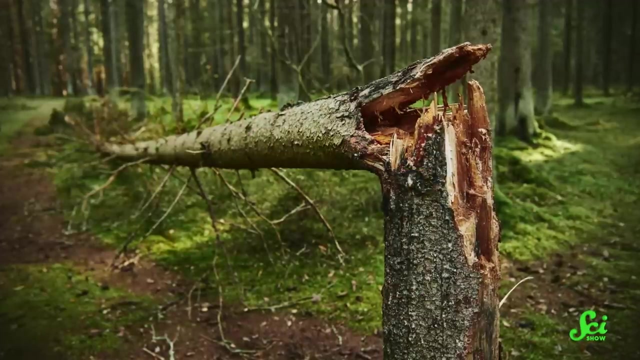 This SciShow video is supported by Brilliant. As a SciShow viewer, you can keep building your STEM skills for 20% off an annual premium subscription at Brilliantorg. slash SciShow. If a tree falls in a forest and doesn't decompose, what happens to it? 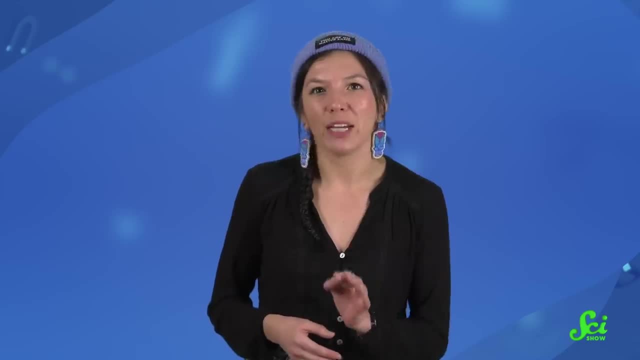 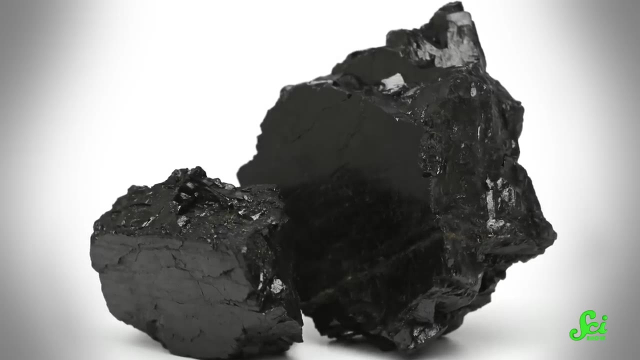 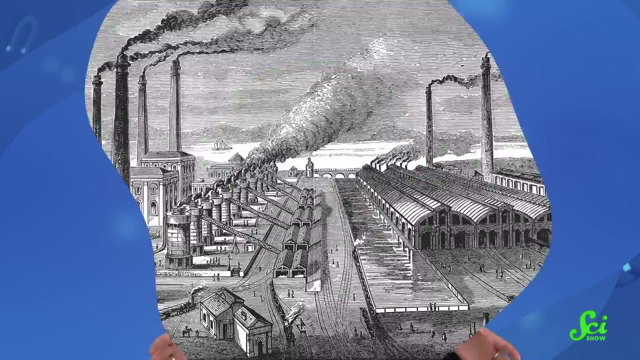 Well, like all living things on Earth, trees are mostly made of carbon, And if that tree happened to exist some 300 million years ago, that carbon might have turned into coal. In fact, we can thank ancient fallen forests for essentially the world's entire supply of coal. 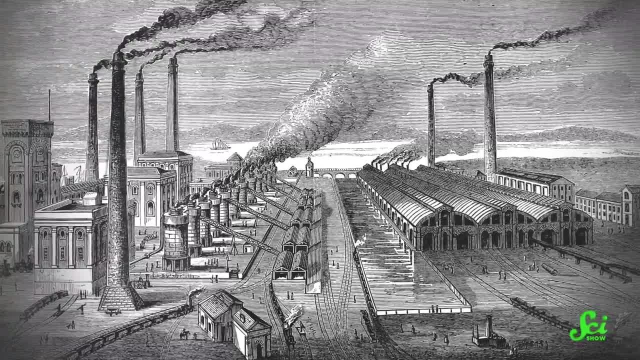 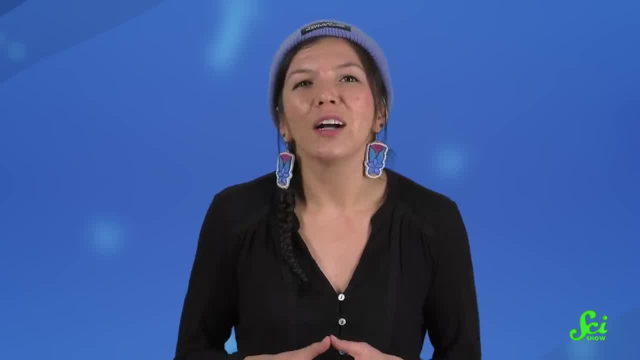 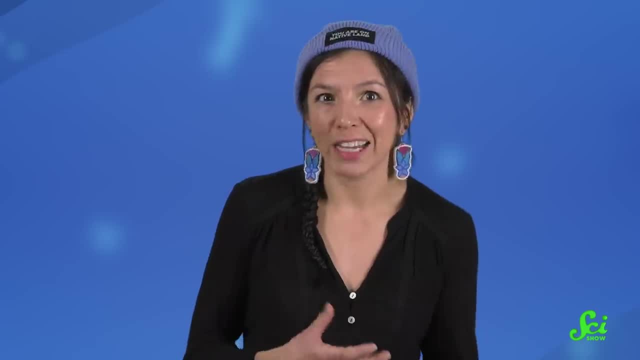 The burning of which made things like steam engines and the entire Industrial Revolution possible. Of course, it has also caused some serious climate problems, And while we look to uncover some of the secrets of these coal-forming forests, we can also focus our efforts on getting that carbon out of the atmosphere. 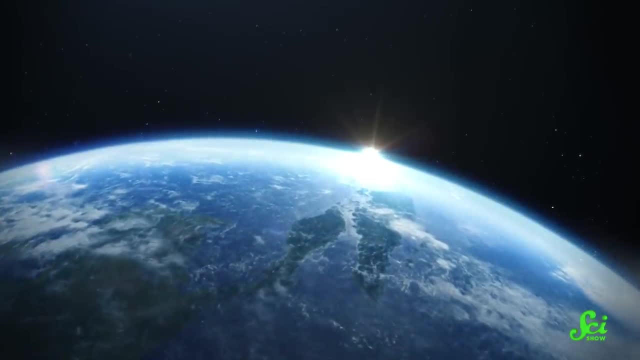 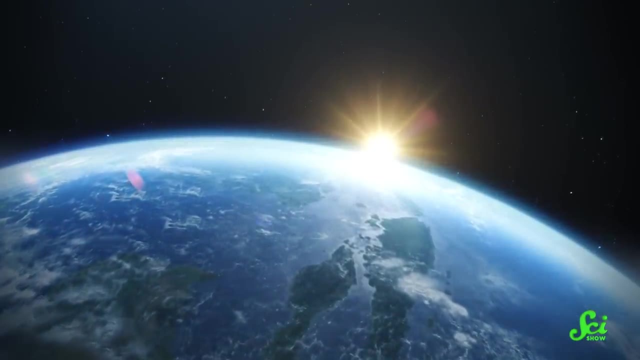 and back where it came from. Carbon is vital to all life on Earth. We find it everywhere, from bodies of living organisms to the seawater and Earth, and in our atmosphere as carbon dioxide, And it's always moving through these forms, through what's called the carbon cycle. 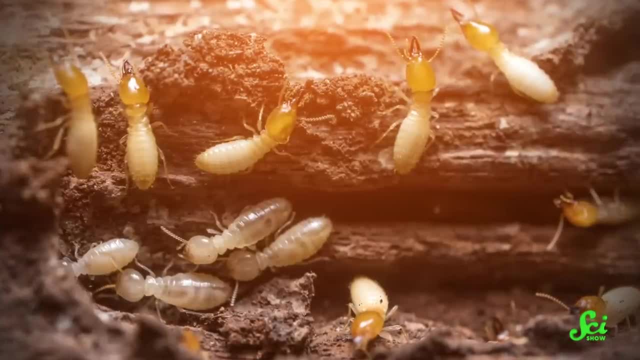 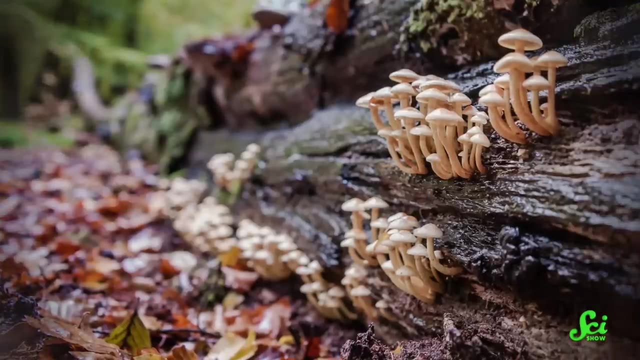 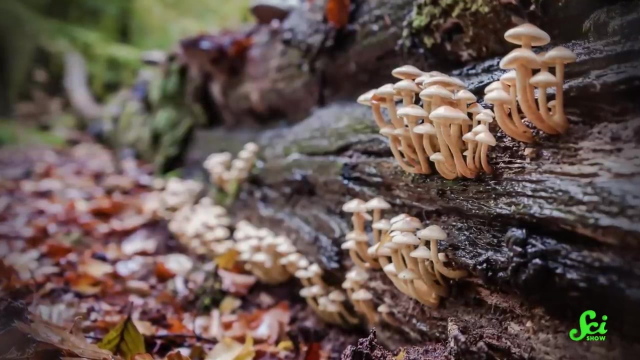 When an organism, like a tree, dies, it's slowly broken down by decomposers, which are other organisms that are specially adapted to eat dead stuff. Fungi are the dominant decomposers, but microorganisms and insects that are adapted to chow down on the dead stuff can also do a lot of heavy lifting. 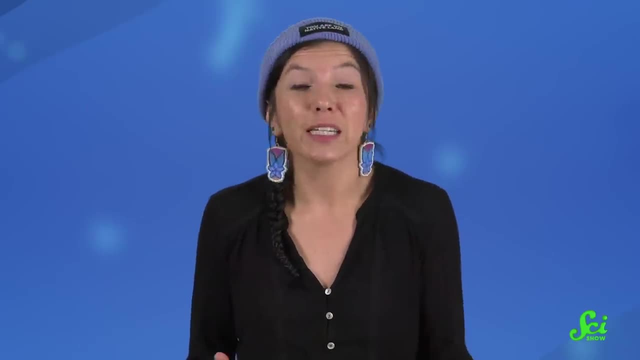 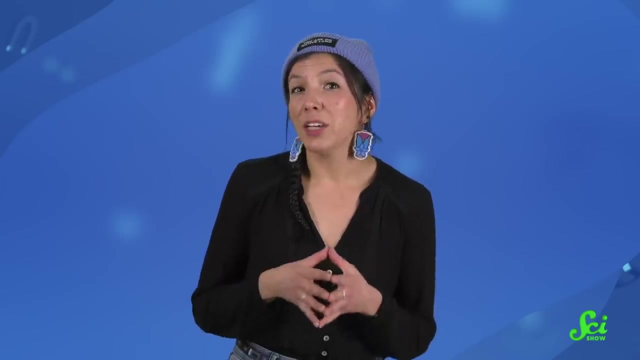 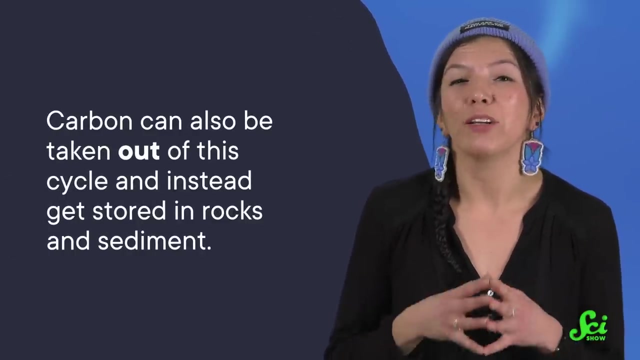 Together they break down tissues and over time release the carbon in them back into the atmosphere to be carbon dioxide gas again. But it turns out that's not the only fate of carbon in dead things, That carbon can also be taken out of this cycle and instead get stored in rocks and sediment. 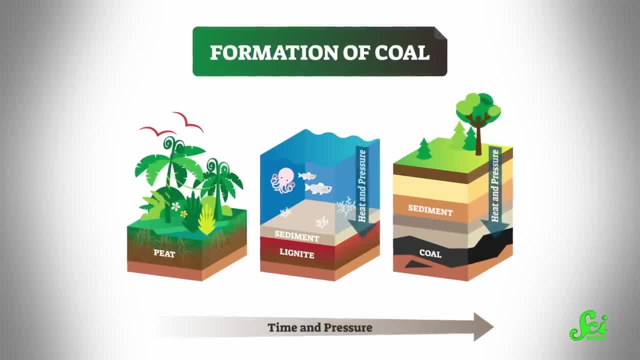 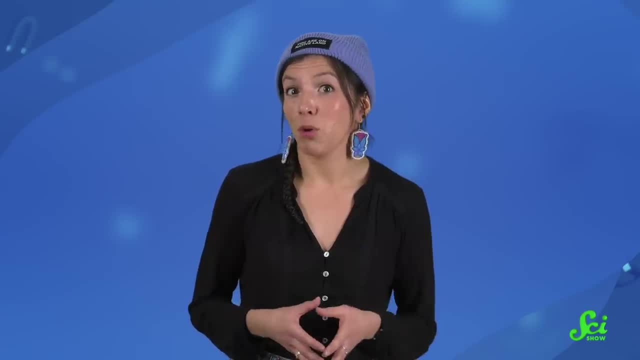 Case in point: coal. Coal forms when carbon from organic matter accumulates in layers that are compressed over millennia into rock, And it turns out that the vast majority of the world's coal formed during a single geologic time period that started about 360 million years ago. 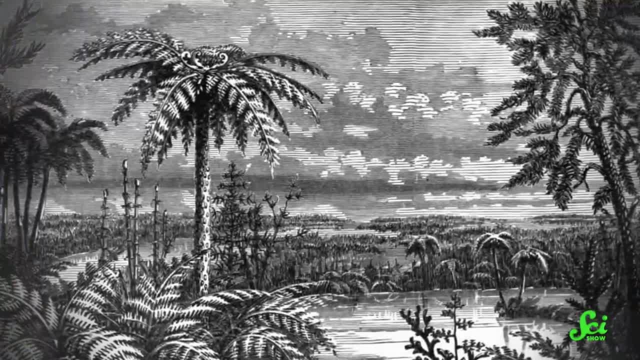 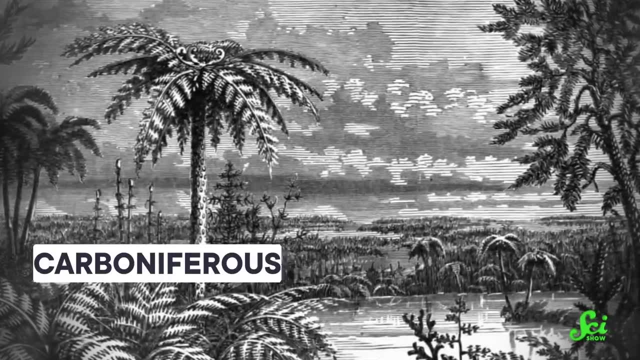 So much coal formed in this period that geologists literally named it after the amount of carbon dating to this time, which is where we get the name carboniferous Coal- really piled up, because the trees and other plant life just flat out didn't break down. And there's never been a time since then where so much coal formed all at once in lots of different places. So what gives? Let's look back at the carboniferous period to find out. Most of the world was pretty tropical at that time. Mild, humid environments were regularly flooded by the surrounding warm ocean waters, and swamp forests reigned supreme, And these swamps saw the rise of the first towering trees, but not the kind of trees we're used to today. They're in a group of plants called lycopsyds. 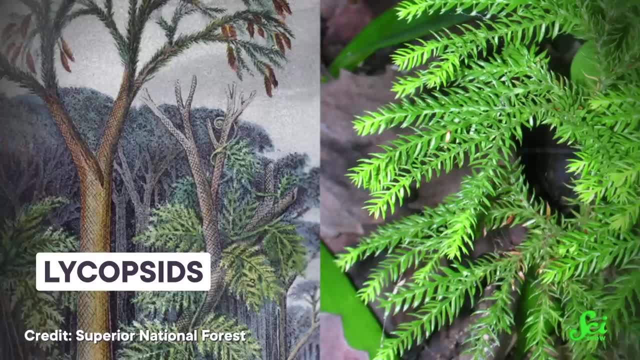 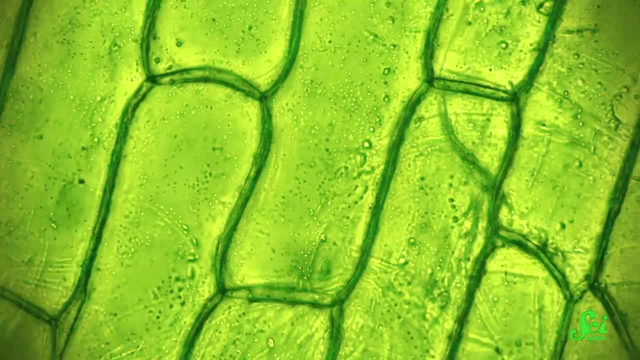 and while today's lycopsyds are only a few inches tall at most, their carboniferous ancestors grew upwards of 35 meters tall. These plants also contained a fibrous tissue called lignin, which gives modern-day plants their rigid structure. 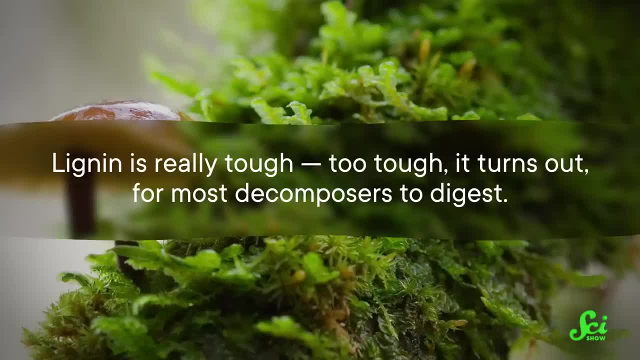 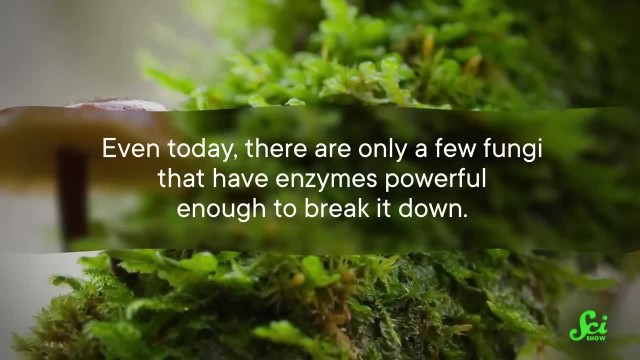 Lignin is really tough, Too tough, it turns out, for most decomposers to digest. Even today, there are only a few fungi that have enzymes powerful enough to break it down. So for a long time scientists thought that fungi simply hadn't yet evolved the ability. 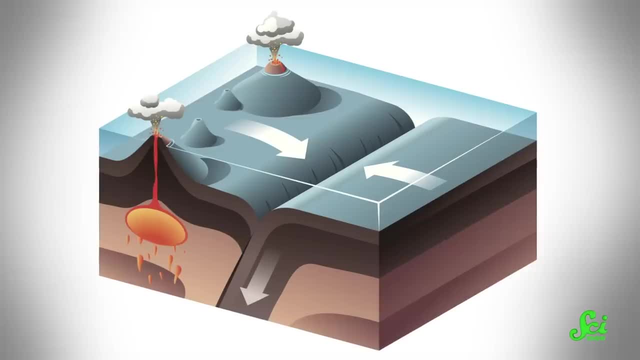 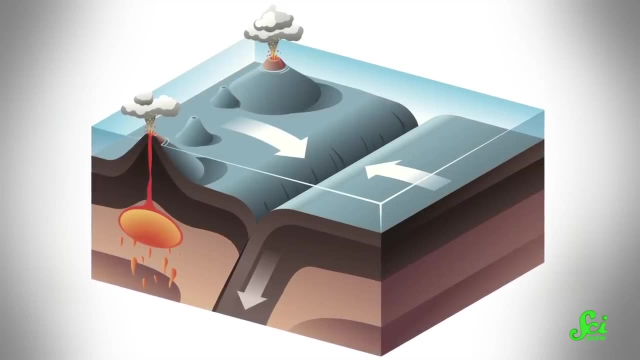 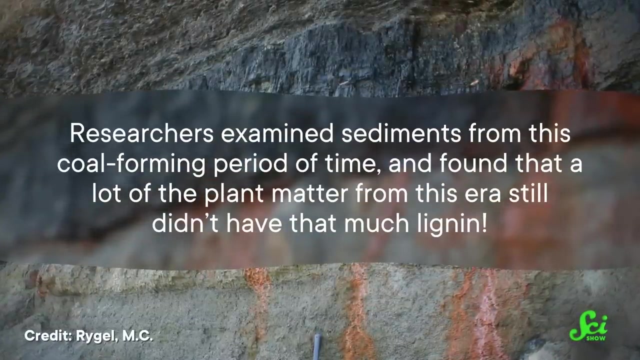 to break down the new woody fibers of plants yet, But in 2016, researchers instead proposed that tectonic plate movement was more likely the influence of coal formation. They examined sediments from this coal-forming period of time and found that a lot of the plant matter from this era still didn't have that much lignin. 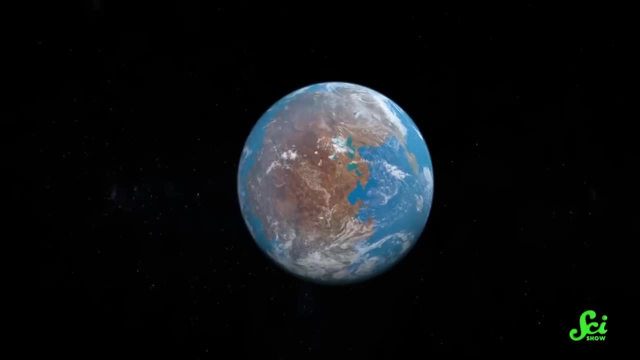 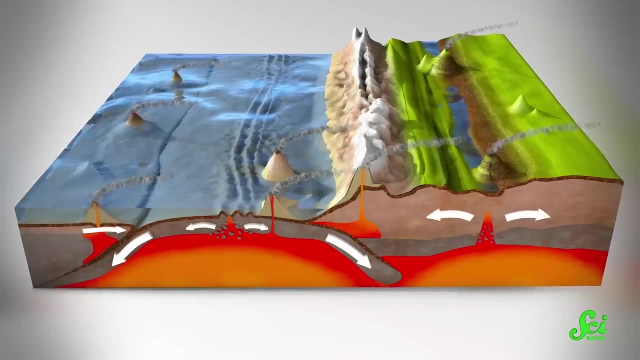 And there was a ton of geologic activity at that time, moving around landmasses that would eventually combine into what we know as Pangea. This plate movement created tall mountains and deep valley basins, which were the perfect places for plant debris to accumulate in mass. The already humid environment was subject to regular flooding, causing the formation of thick marshy layers. When you're at the bottom of a waterlogged swamp, you won't find much oxygen around, And one of the key ingredients of decomposition is oxygen. So, lignin or not, the fact that these swamps sealed out oxygen? 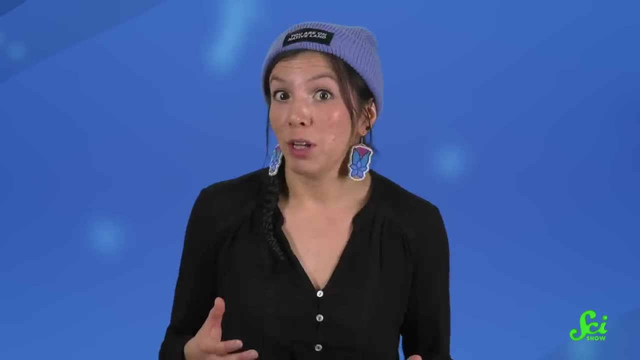 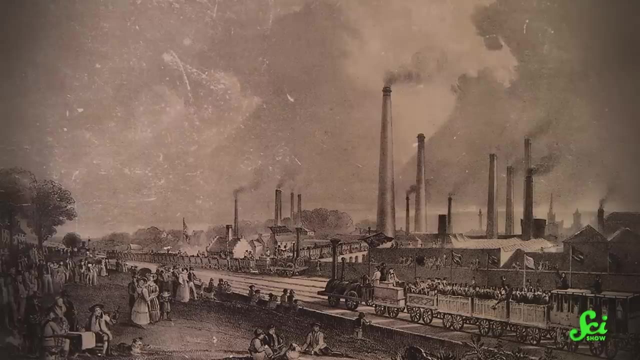 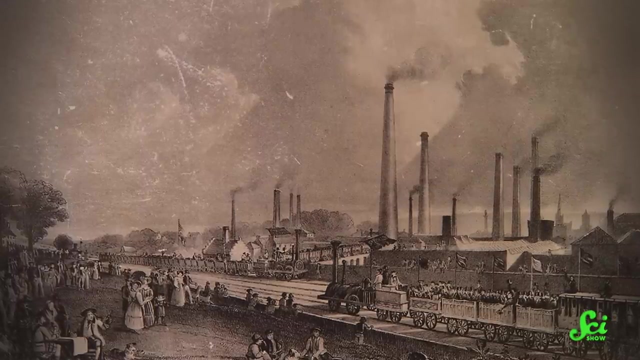 protected the plant matter from decomposing, Given a few million years, all that carbon compressed down to form the coal we know and burn today. We humans have been burning coal for thousands of years, But coal really became important during the Industrial Revolution when we used it to power steam engines and other technologies. 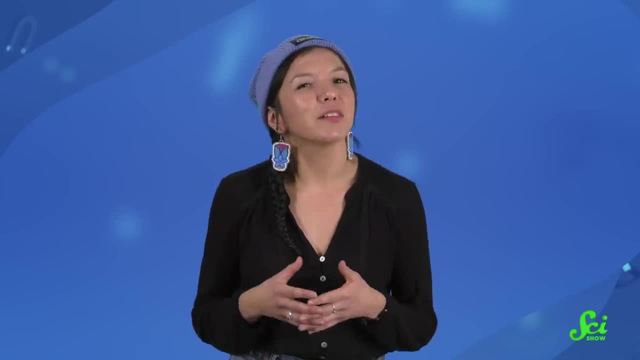 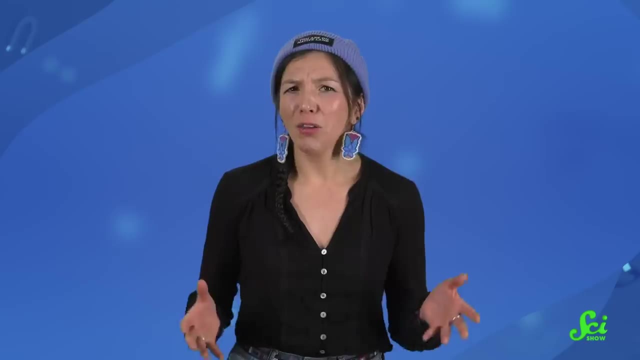 That made manufacturing easier, but it solidified our dependence on fossil fuels And it's now one of the biggest contributors to our warming climate. All that coal is now in the air And it's now one of the biggest contributors to our warming climate. All that coal is now in the air. All that coal was once a carbon sink. For millions of years it kept the trapped carbon locked away and out of the carbon cycle. By burning it, we're adding much more carbon into the atmosphere than would be there otherwise. 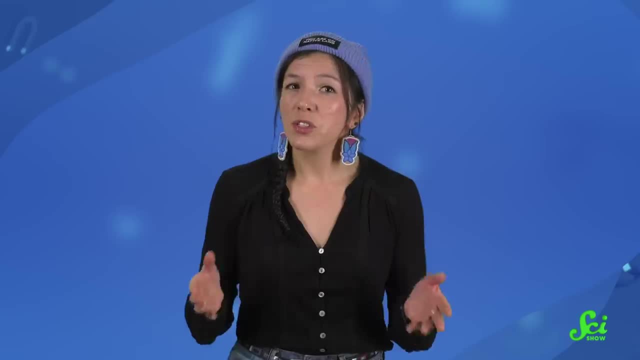 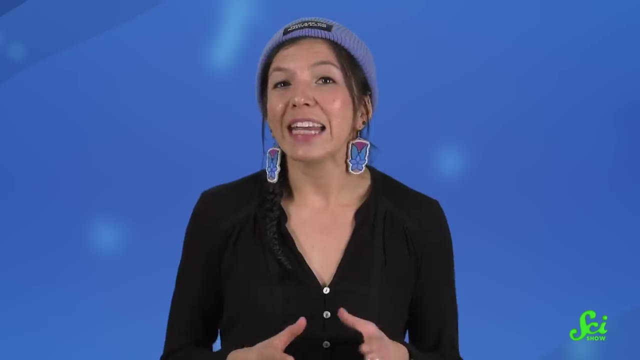 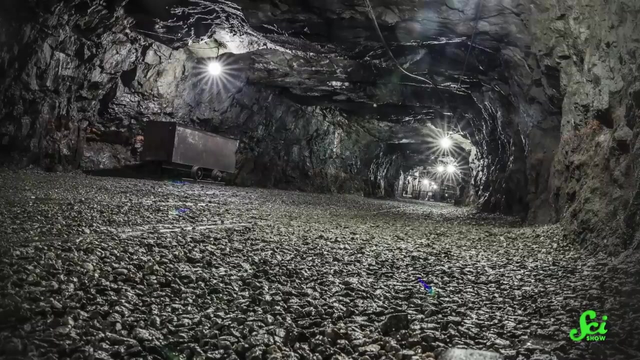 All way faster than decomposers ever could have done. So as we try to find solutions to the climate crisis, we're going to have to stop burning so much carbon. But in thinking of other ways to mitigate the amount of carbon in our atmosphere right now, we can also take some inspiration from the Carboniferous Period and start to sequester it too. Of course we can't rely on natural coal formation to happen at the scale it was during the Carboniferous Period. The conditions are too different today from what was going on back then. 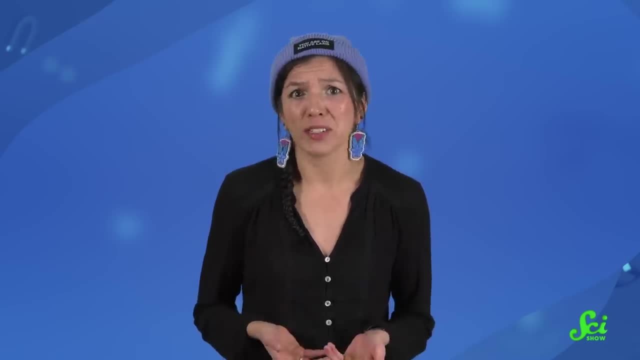 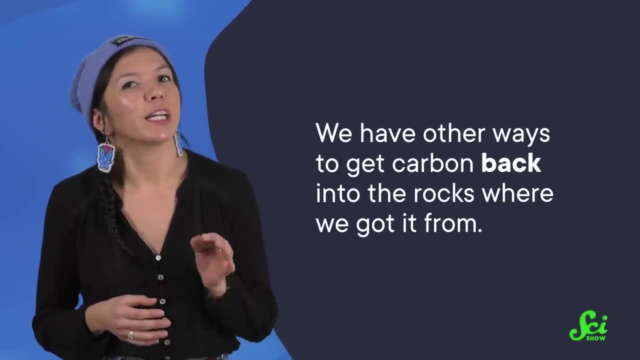 not that it would even happen on a timescale that will help us. We just don't have the millions of years to spare. But it turns out we have other ways to get carbon back into the rocks where we got it from: geologically isolating it and keeping it out of our atmosphere. 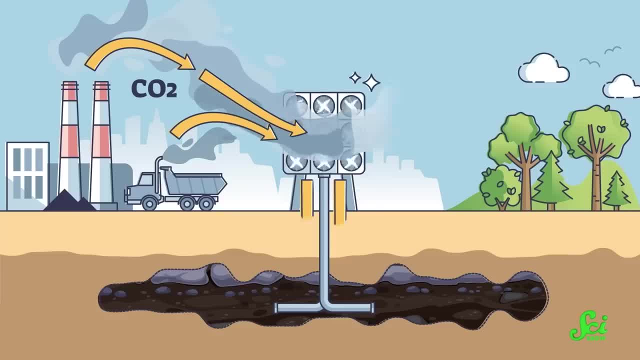 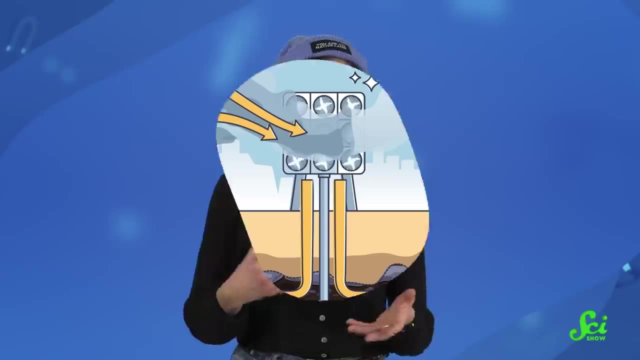 Basically, we can inject it into rocks in the form of carbon dioxide. Rock types with certain minerals containing calcium, magnesium and iron are the best candidates for this process, since those elements will react with carbon dioxide to help lock it in place. It's not exactly a straightforward solution, since these processes aren't easy to pull off. 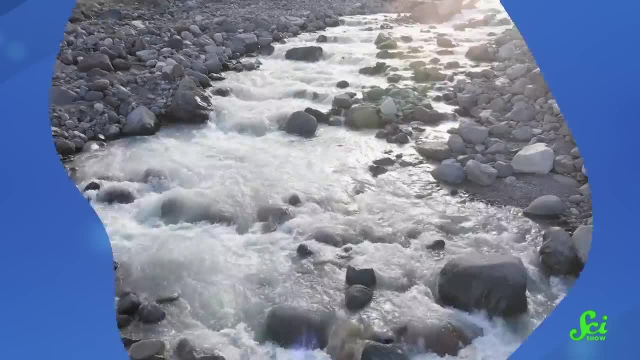 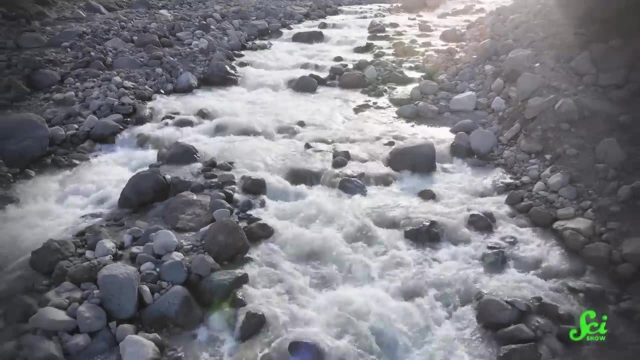 and they can be very costly. Plus, there are potential risks. Some studies have shown that chemical reactions within the rocks can cause the carbon dioxide to find its way back into the atmosphere and even into our drinking water, And not in a fun fizzy water kind of way. 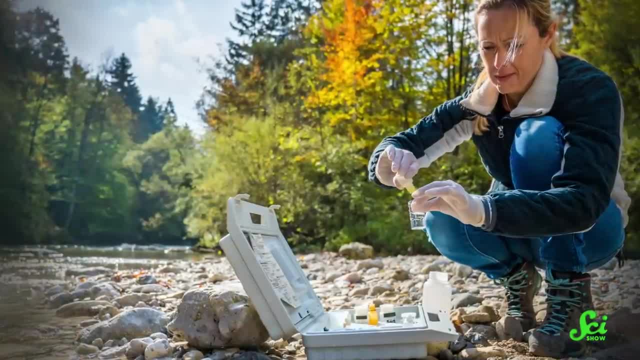 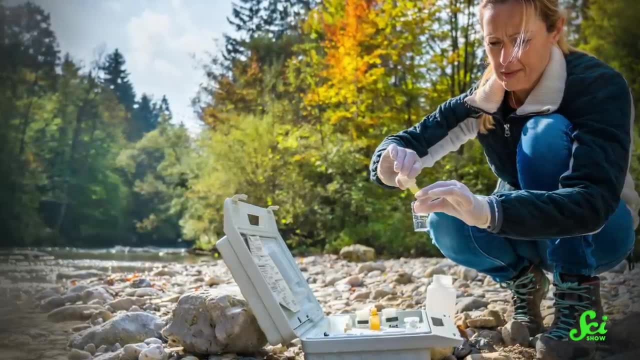 Excess carbon dioxide in water systems can increase the amount of dissolved solids in the water, which affects the taste. It can also make the water more acidic and could even increase the metals present. Other research has shown that if we pump that carbon into the wrong locations, 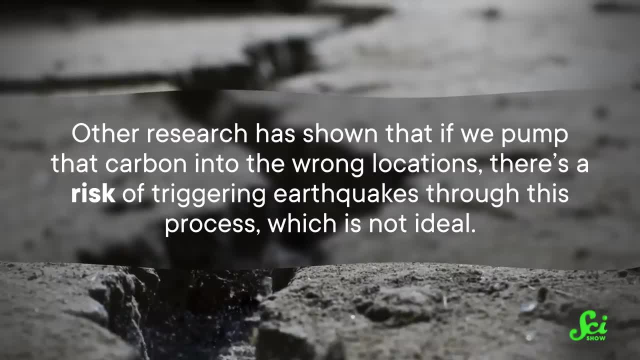 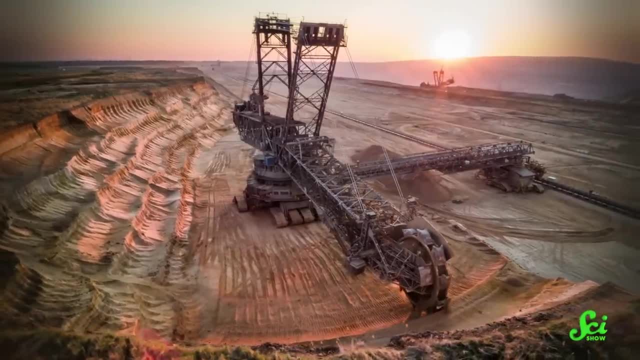 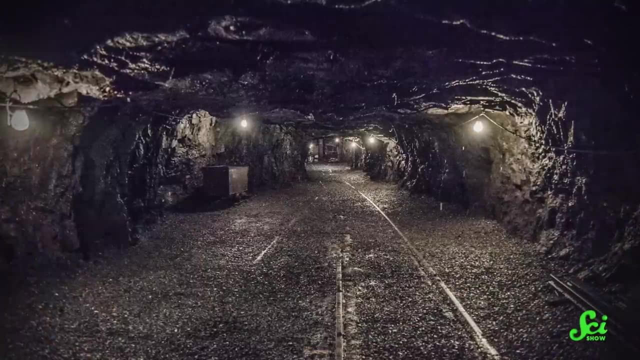 there's a risk of triggering earthquakes through this process, which is not ideal. So what locations are we looking for? Well, it's looking like areas where we've already extracted coal and oil are actually best suited to the process. See, when it comes to geologic activity like earthquakes. 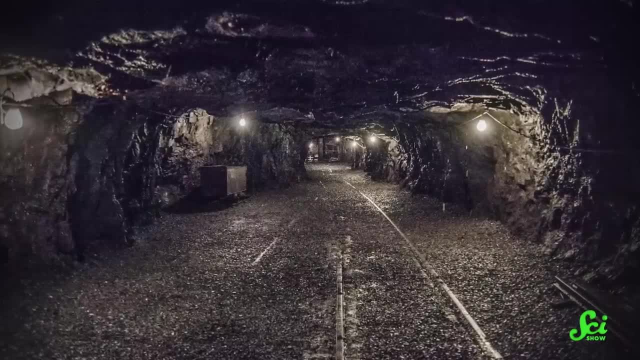 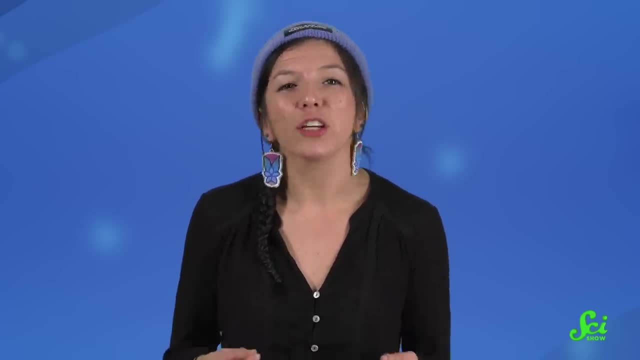 areas that are chosen for mining tend to be more quiescent or dormant, So areas where we've extracted resources already may be better candidates for carbon sequestration, just because of that fact. So it does look like one day- large-scale geologic carbon storage. 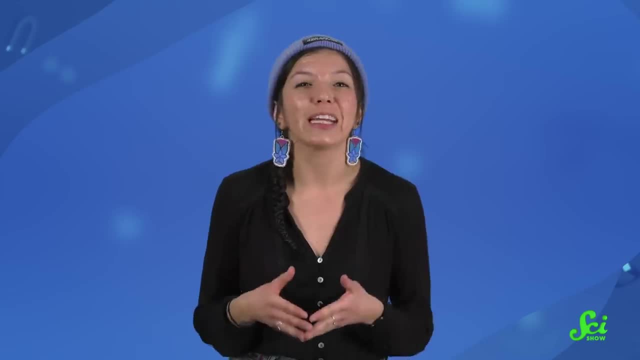 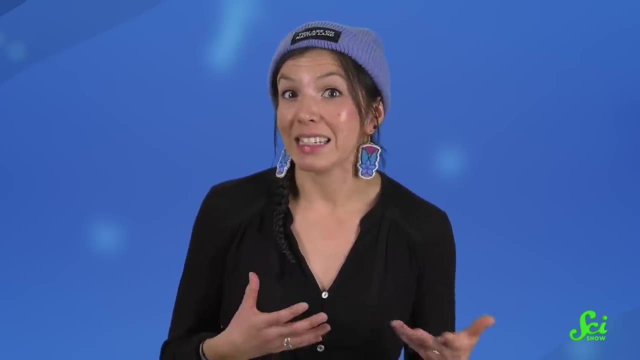 could be one of the solutions we can use. We can mobilize in an effort to gain control of our massive climate problem, Even if we have a long way to go before we can store carbon deep in the rocks at the scale that ancient forests did. we can thank the Carboniferous Forest for two things.